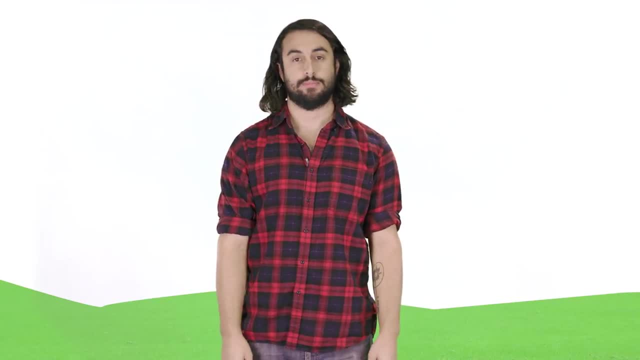 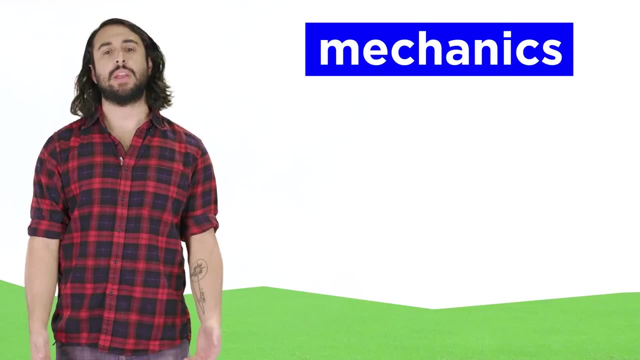 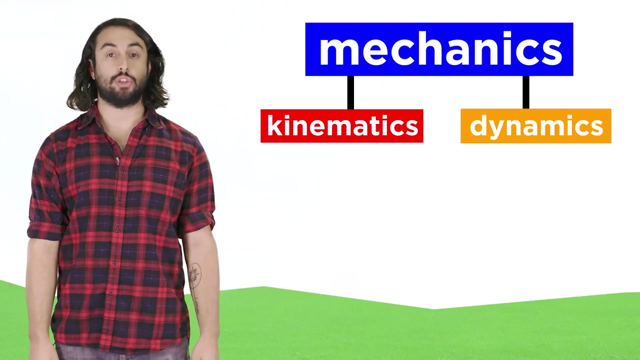 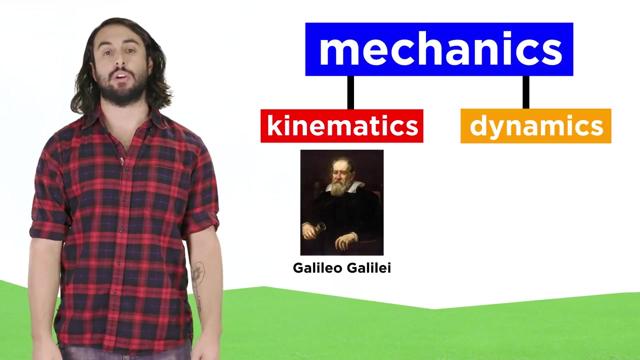 Hey, it's Professor Dave. let's talk about horizontal motion. As we learn classical physics, a big topic of study will be mechanics. This is a branch of physics that can be divided into two smaller topics: kinematics and dynamics. Kinematics, which was developed largely by Galileo in the early 1600s, deals with equations. 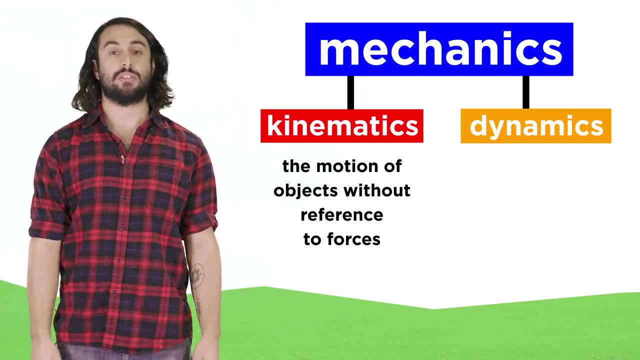 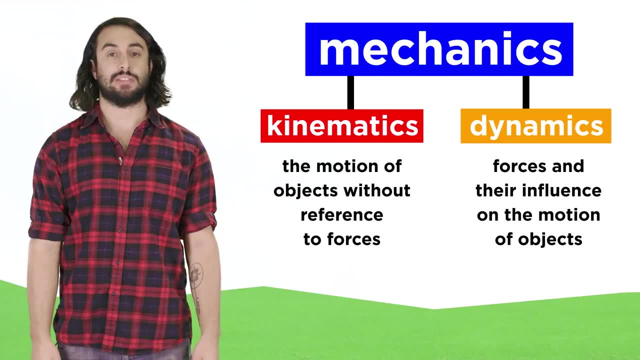 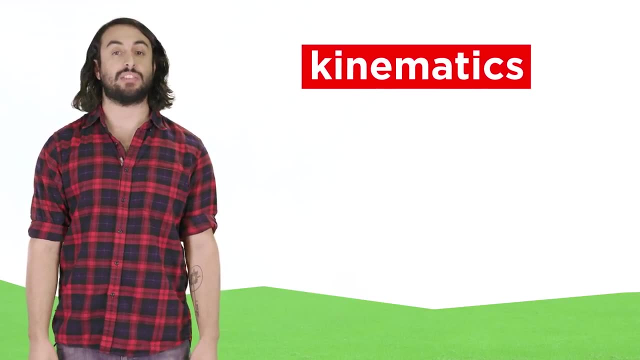 that describe the motion of objects without reference to forces of any kind, whereas dynamics is the study of the effect that forces have on the motion of objects. These topics together comprise mechanics. We are going to focus on kinematics over the next few tutorials so that we can familiarize. 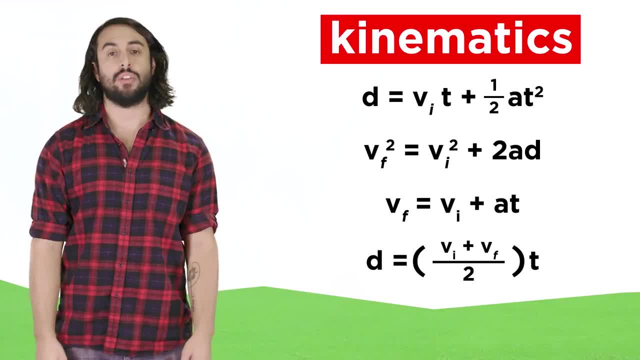 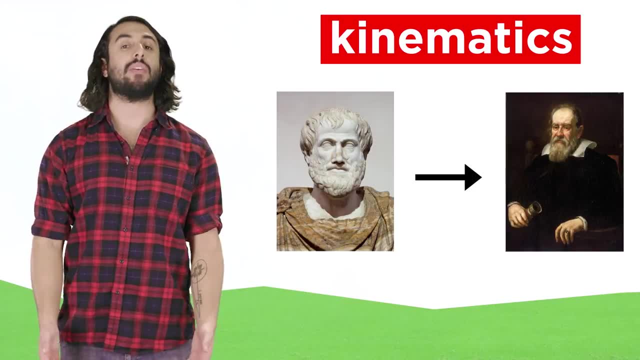 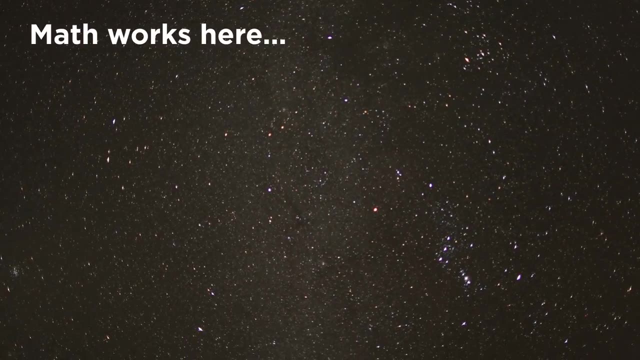 ourselves with the ways that simple equations will govern the motion of objects in one and two dimensions. These equations are revolutionary Because from Aristotle until Galileo, we thought that mathematics could only describe the perfect motion of divine celestial objects and that the motion of objects on earth was 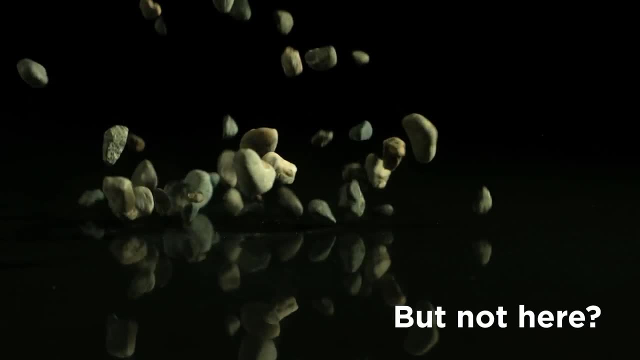 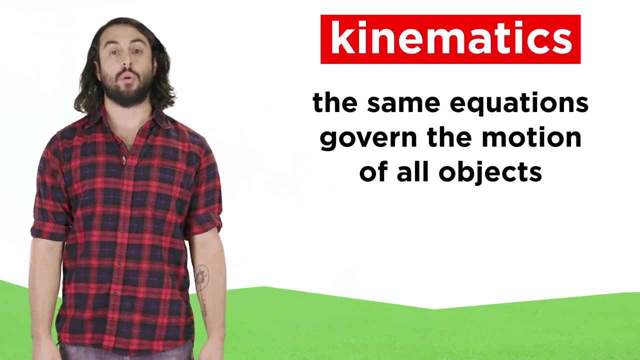 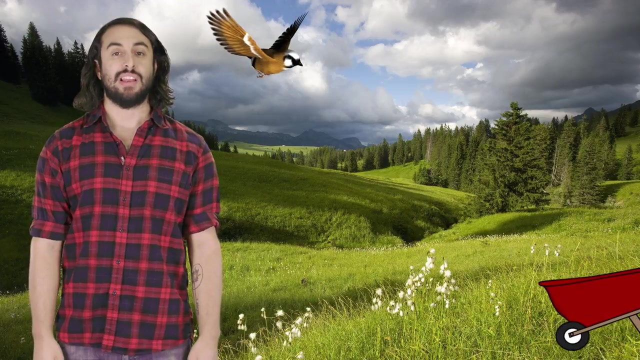 too imperfect and unpredictable to calculate. But we soon found that the same equations govern the motion of all objects, whether on earth or in space. It is simply that on earth we must make approximations, since there are a greater number of variables. 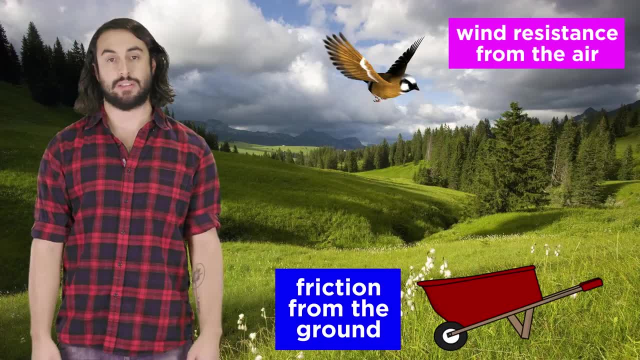 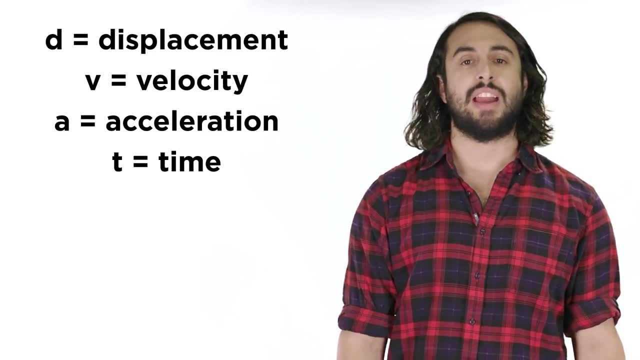 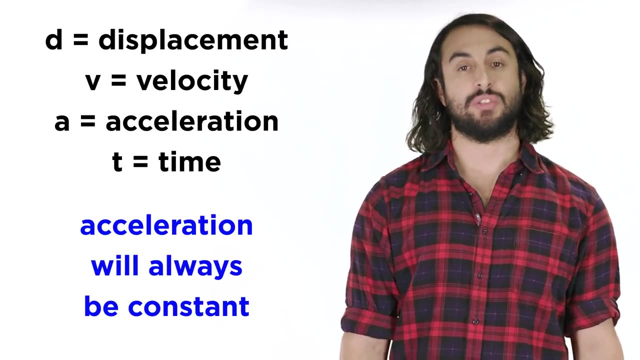 such as direction and atmosphere, that affect motion in various ways. The kinematic equations include variables for displacement, velocity, acceleration and time, And, in the context of kinematics, acceleration will always have a constant value, whether positive, negative or zero, since we won't look at forces that could cause acceleration. 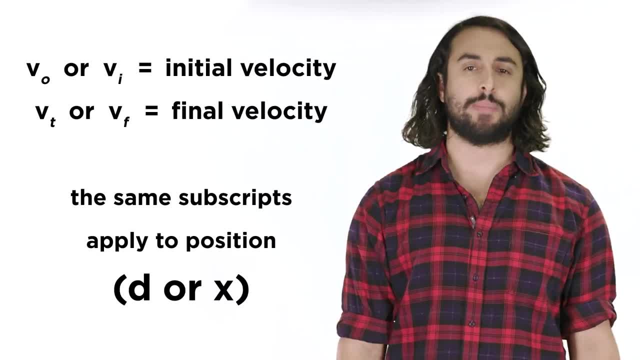 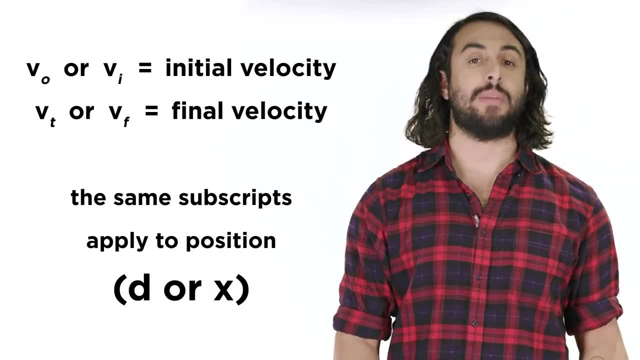 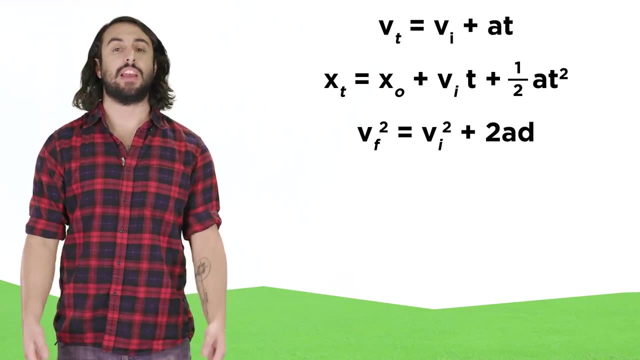 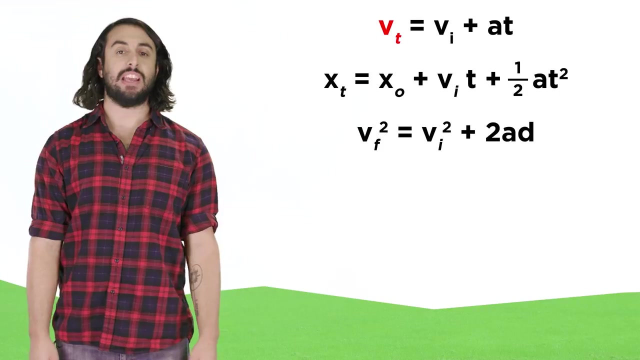 to change over time. When you see a subscript of zero after velocity or displacement, it indicates the initial conditions which will have some implication, depending on the problem we are looking at. Here are the three fundamental kinematic equations we will be using. The first one says that the velocity of an object at any time, t, is equal to the initial. 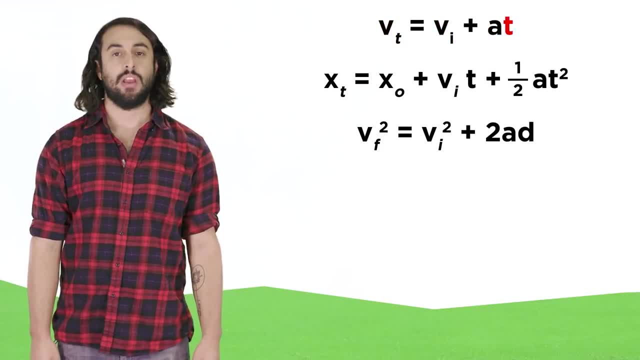 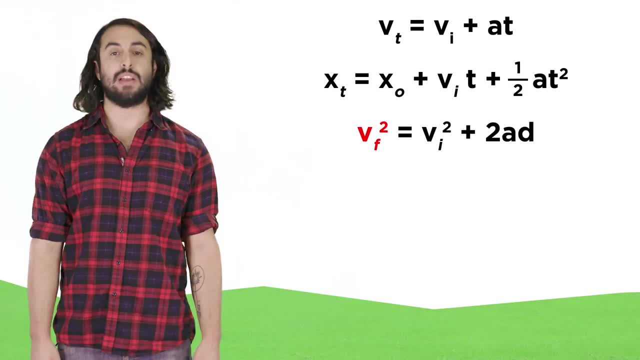 to its initial position plus the initial velocity times time. The next one says that the position of an object with respect to a point of origin will be equal to its initial position plus the initial velocity times time. The next one says that the position of an object with respect to a point of origin will be equal. 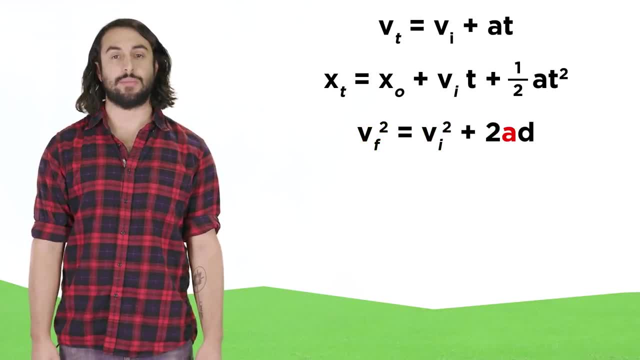 to its initial position plus the initial velocity times time. The next one says that the position of an object with respect to a point of origin will be equal to its initial position plus the initial velocity times time. The next one says that the position of an object with respect to a point of origin will be equal. 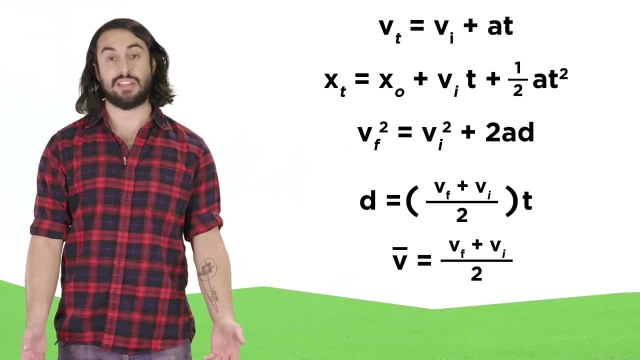 to its initial position plus the initial velocity times time. The next one says that the position of an object with respect to a point of origin will be equal to its initial position plus the initial velocity times time. The next one says that the position of an object with respect to a point of origin will be equal. 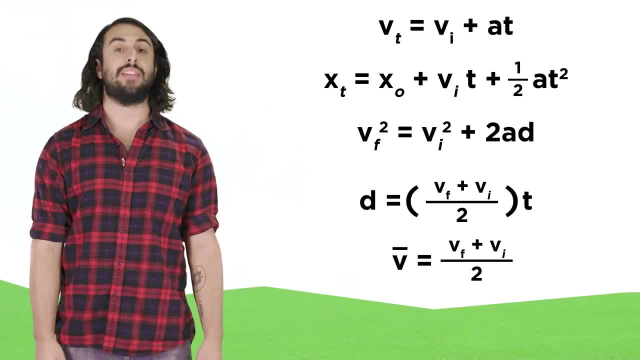 to its initial position plus the initial velocity times time. The next one says that the position of an object with respect to a point of origin will be equal to its initial position plus the initial velocity times time. The next one says that the position of an object with respect to a point of origin will be equal. 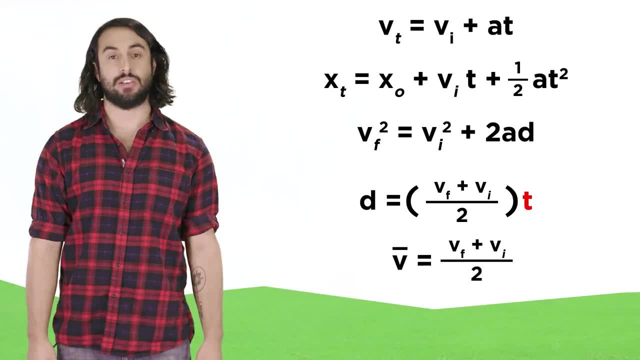 to its initial position plus the initial velocity times time. The next one says that the position of an object with respect to a point of origin will be equal to its initial position plus the initial velocity times time. The next one says that the position of an object with respect to a point of origin will be equal. 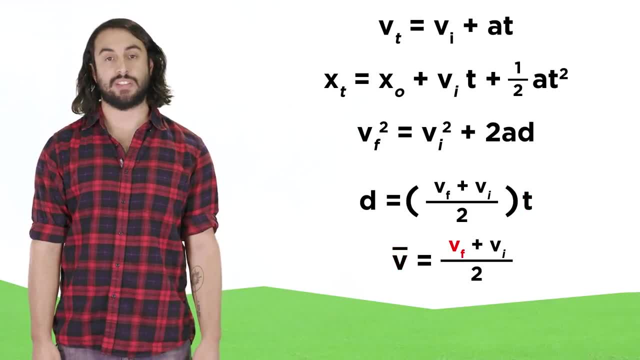 to its initial position plus the initial velocity times time. The next one says that the position of an object with respect to a point of origin will be equal to its initial position plus the initial velocity times time. The next one says that the position of an object with respect to a point of origin will be equal. 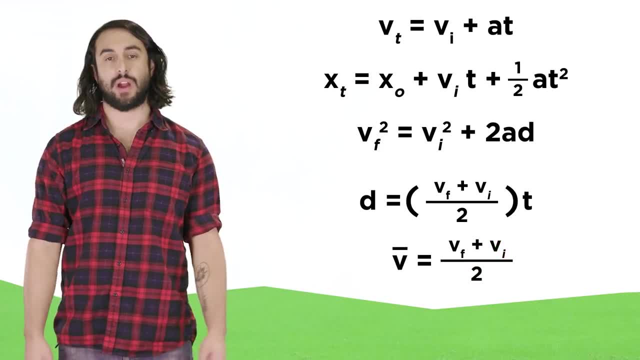 to its initial position plus the initial velocity times time. The next one says that the position of an object with respect to a point of origin will be equal to its initial position plus the initial velocity times time. The next one says that the position of an object with respect to a point of origin will be equal. 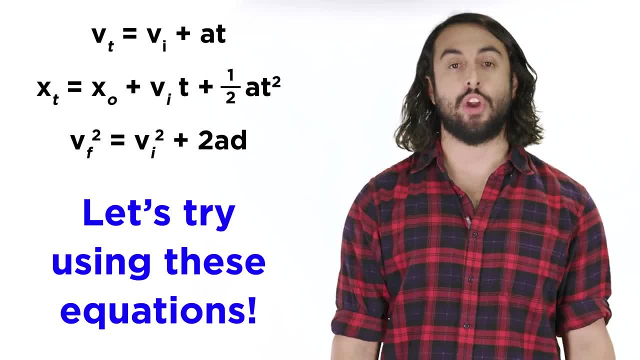 to its initial position plus the initial velocity times time. The next one says that the position of an object with respect to a point of origin will be equal to its initial position plus the initial velocity times time. The next one says that the position of an object with respect to a point of origin will be equal. 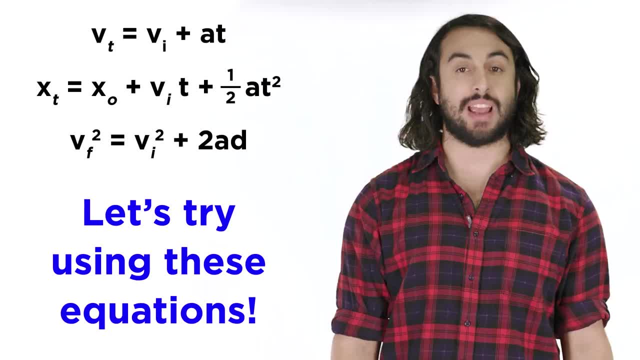 to its initial position plus the initial velocity times time. The next one says that the position of an object with respect to a point of origin will be equal to its initial position plus the initial velocity times time. The next one says that the position of an object with respect to a point of origin will be equal. 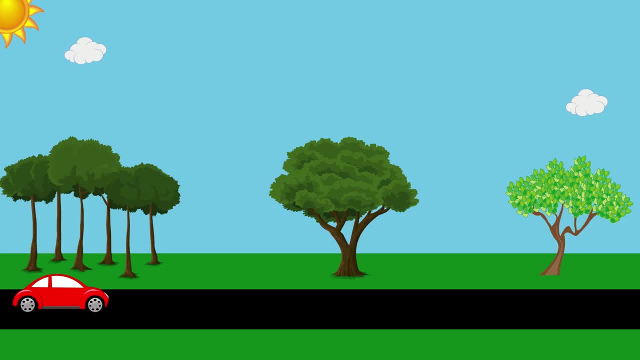 to its initial position plus the initial velocity times time. The next one says that the position of an object with respect to a point of origin will be equal to its initial position plus the initial velocity times time. The next one says that the position of an object with respect to a point of origin will be equal. 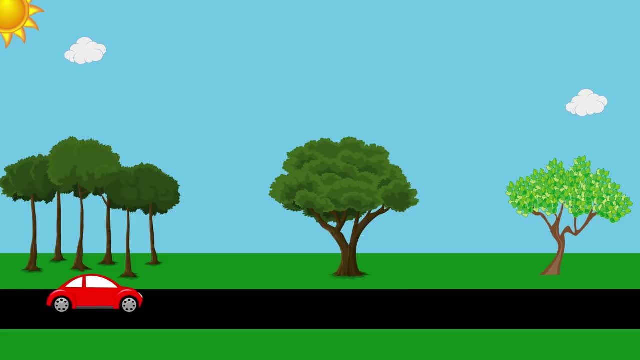 to its initial position plus the initial velocity times time. The next one says that the position of an object with respect to a point of origin will be equal to its initial position plus the initial velocity times time, and apply a constant acceleration of 2.5 meters per second squared. 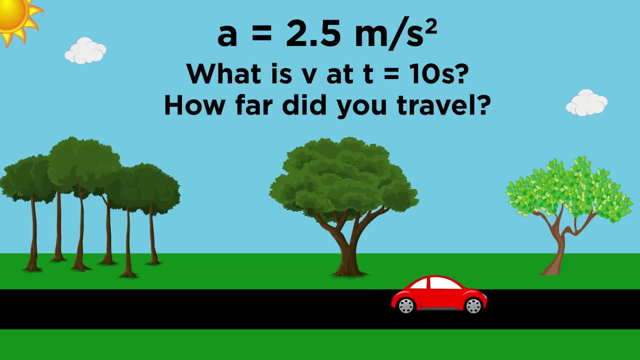 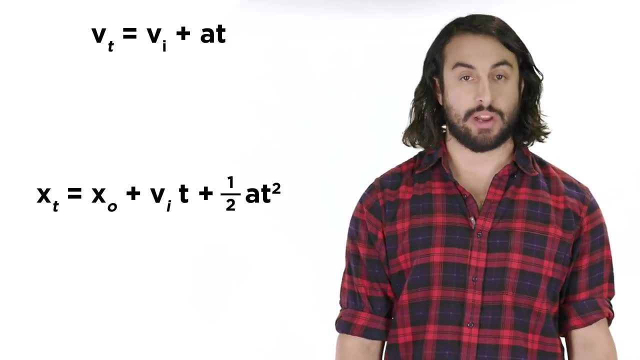 What will your velocity be after ten seconds and how far will you have traveled in that time? We can use these two equations to find the answers. We just have to plug in what we know For the velocity. we know that the initial velocity was zero because we were at rest. 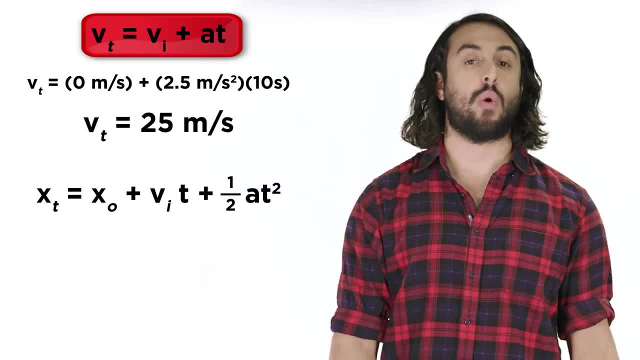 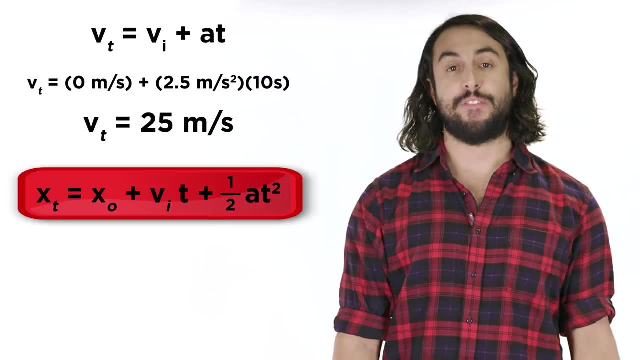 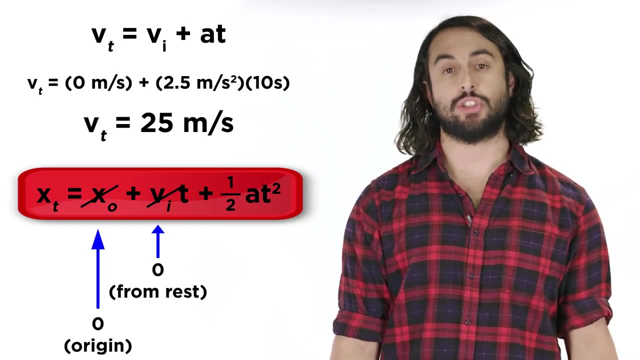 So we just multiply acceleration by time and we get 25 meters per second. That is the velocity of the car after ten seconds. Now to find how far you will have traveled, you will use this equation Once again. initial velocity is zero, so this entire term can be ignored. 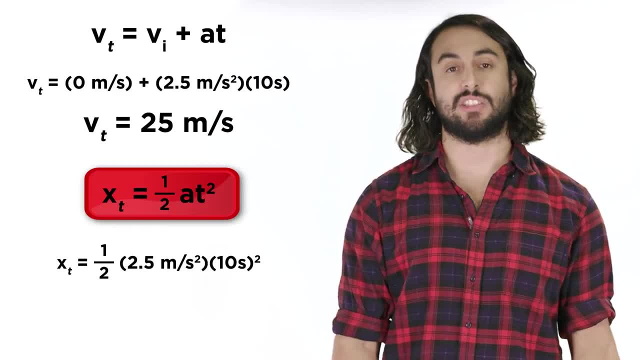 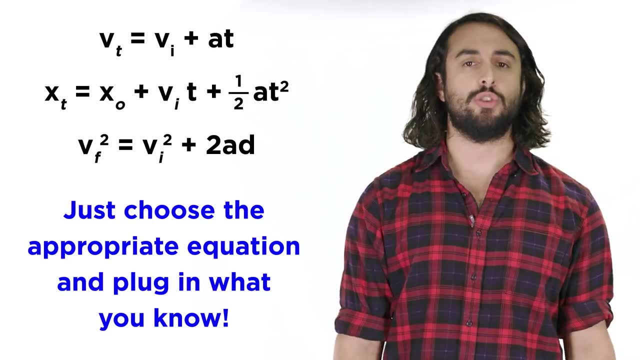 Then we have one half times the acceleration times, ten seconds squared, and we should get 125 meters traveled over this time span. So it really is this simple: you just choose the equation that is appropriate for what you are solving for and plug in what you know. 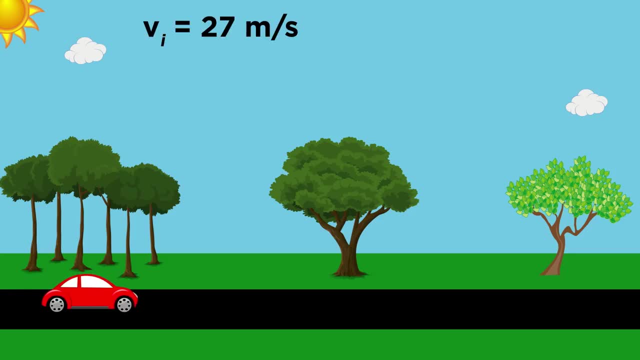 Let's now consider a car that is already in motion with a velocity of 27 meters per second. Let's say you need to stop suddenly, so you press on the brakes, initiating a rapid deceleration of negative 8.4 meters per second, squared. 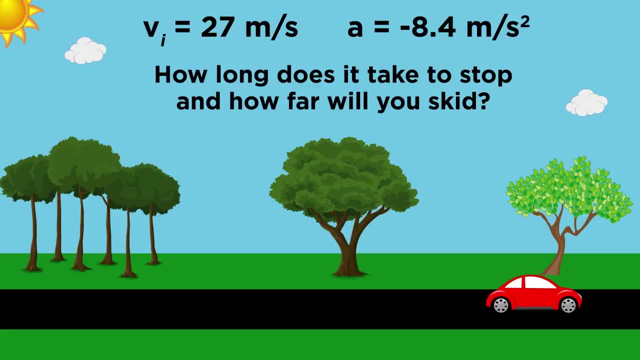 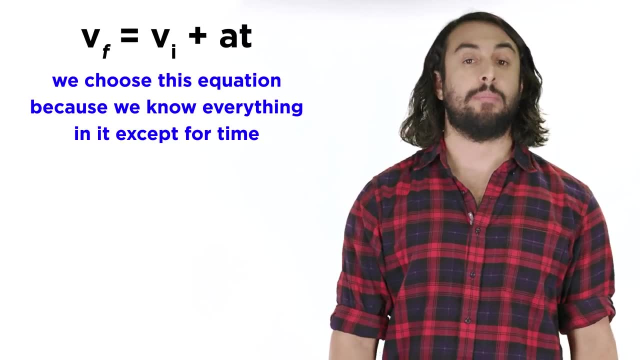 How long will it take the car to come to a stop and how far will it travel while your foot is on the brake? Once again, let's use this equation to solve for time. It must be this equation because we know everything in it. 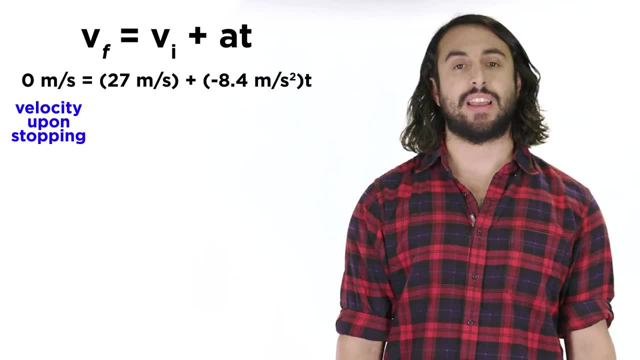 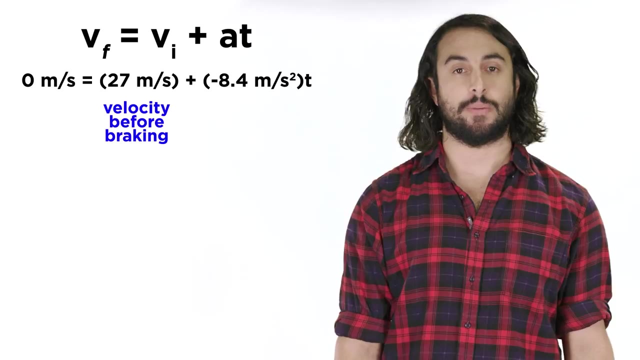 For velocity, let's plug in zero, because we are curious about the time elapsed at the moment that the car stops moving and the velocity when it has stopped moving will be zero. The initial velocity is the 27 meters per second we mentioned and we can plug in the. 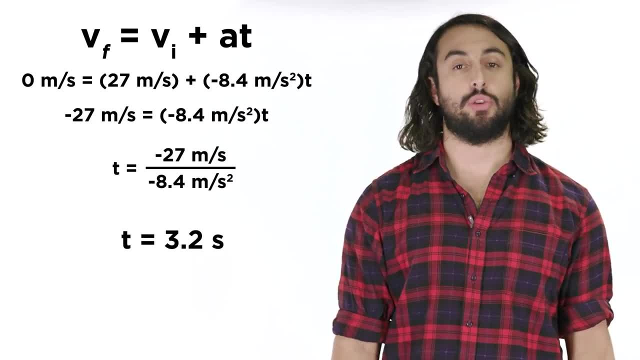 acceleration, solve for time and get 3.2 seconds. Now that we know the time associated with this event, we can use this other equation to find the braking distance. So we can plug in zero and we can solve for time and get 3.2 seconds. Now that we know the time associated with this event, we can use this other equation to find the braking distance. 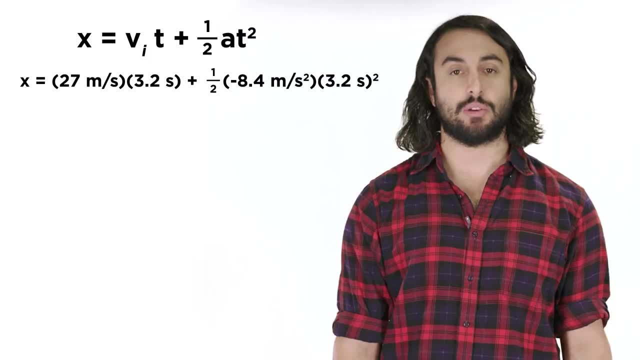 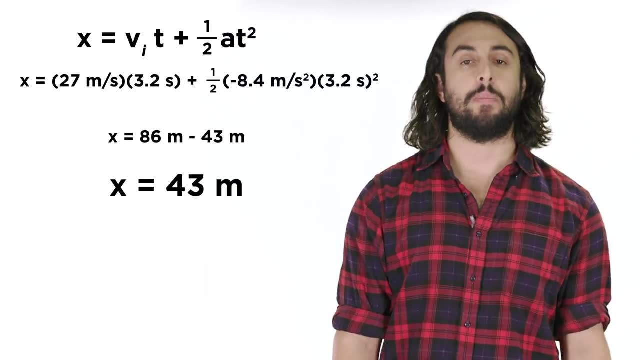 So we can plug in zero and we can solve for time and get 3.2 seconds. We plug in the initial velocity and acceleration we mentioned before, as well as the 3.2 seconds we just calculated and solve for x, which will be about 43 meters traveled from the